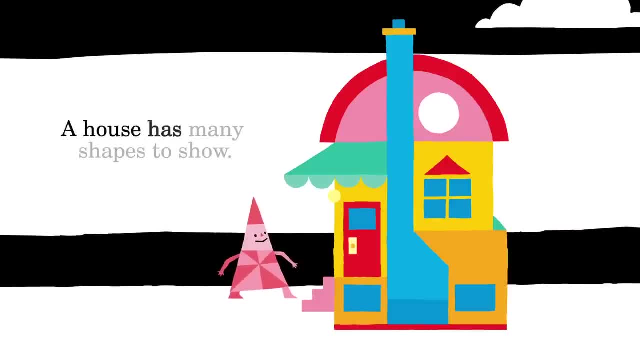 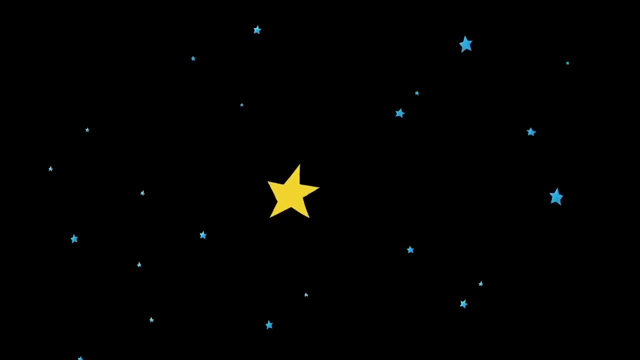 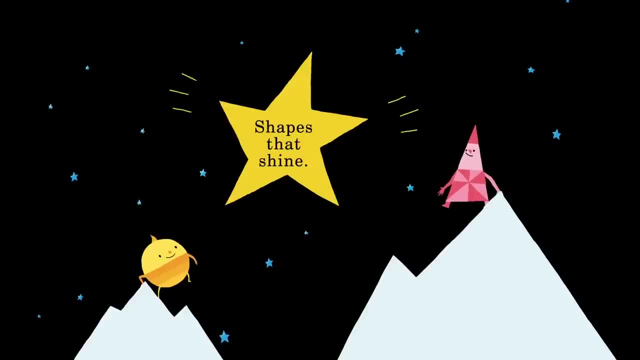 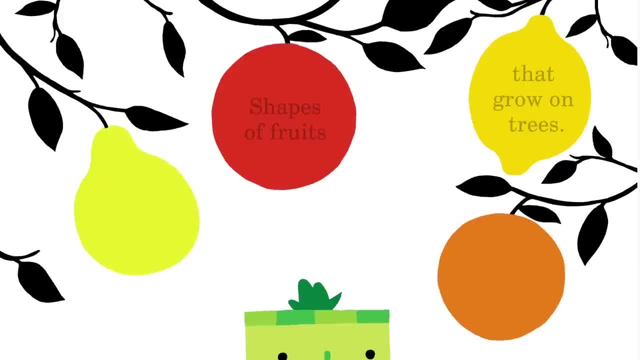 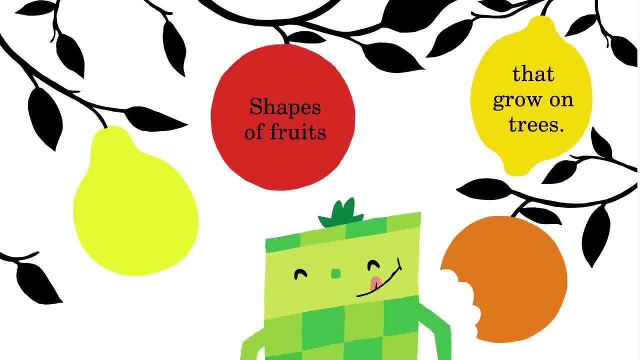 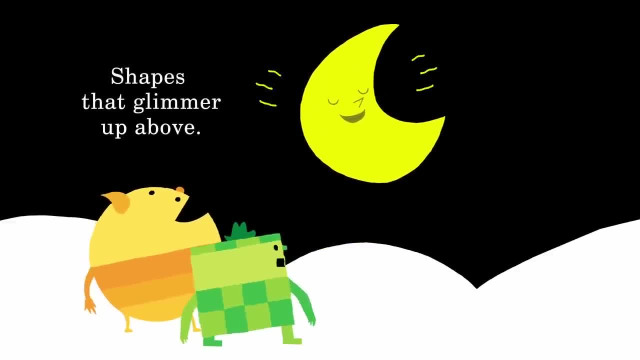 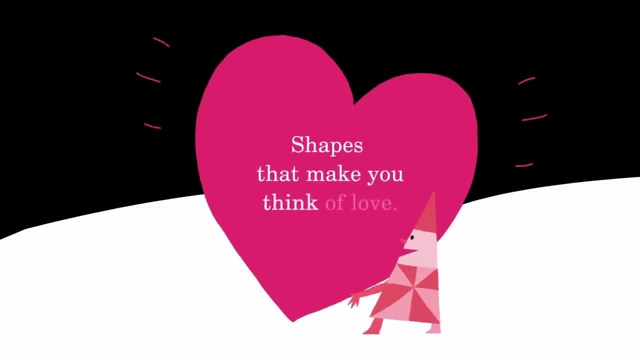 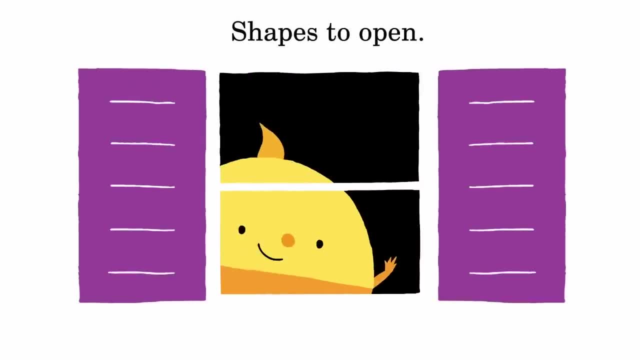 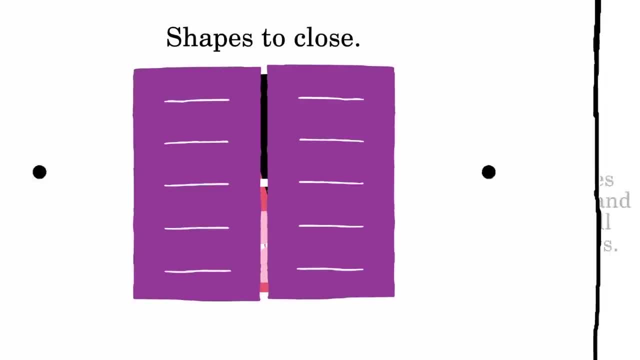 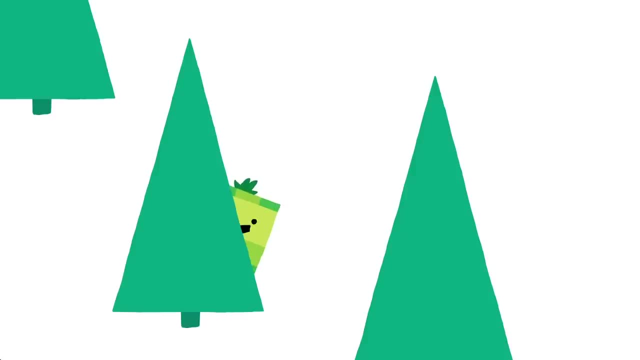 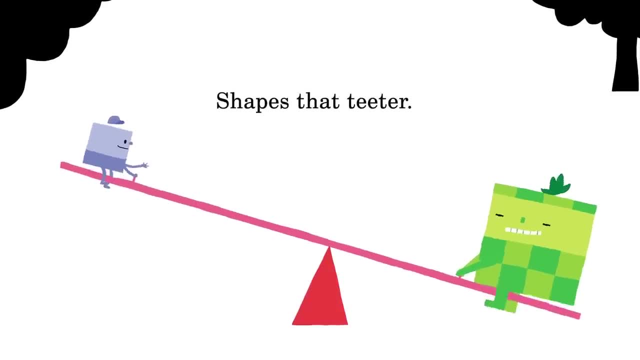 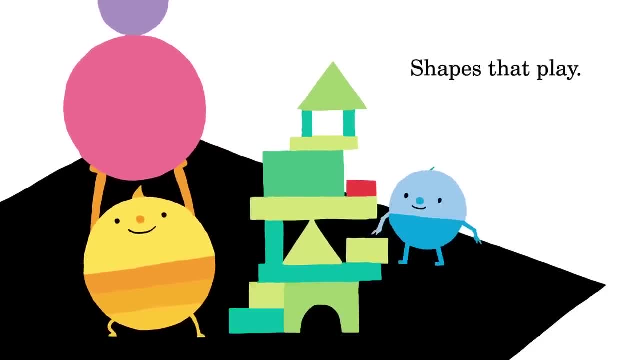 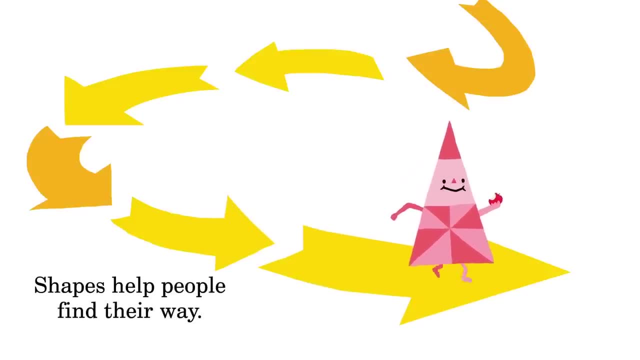 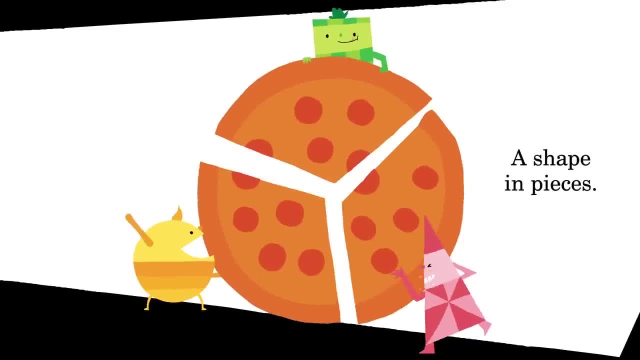 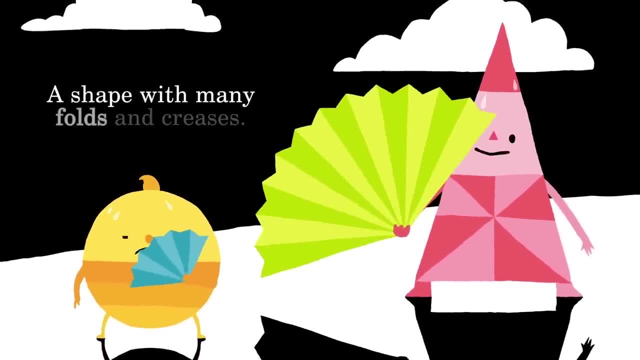 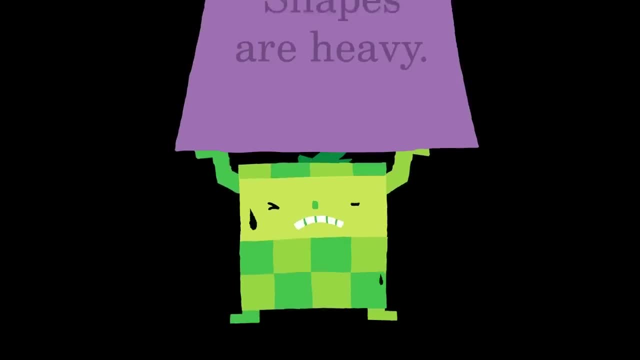 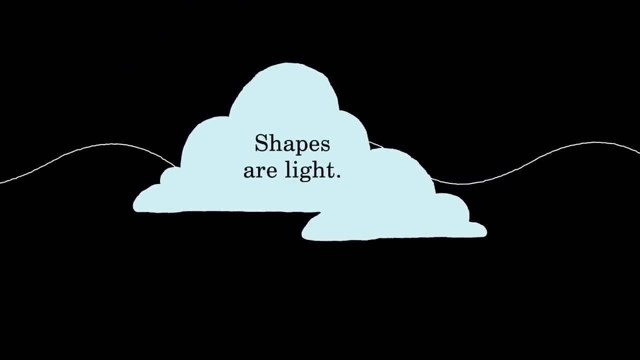 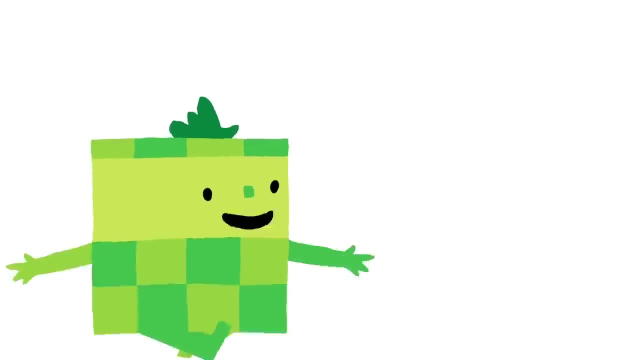 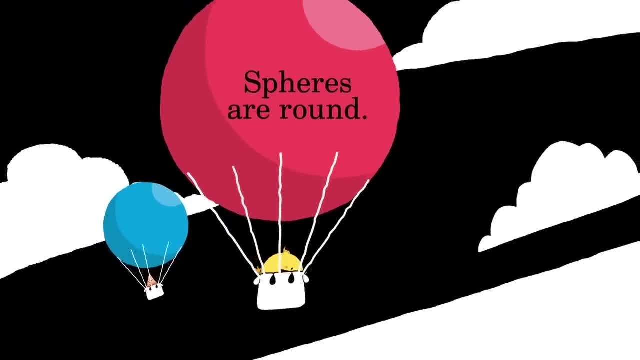 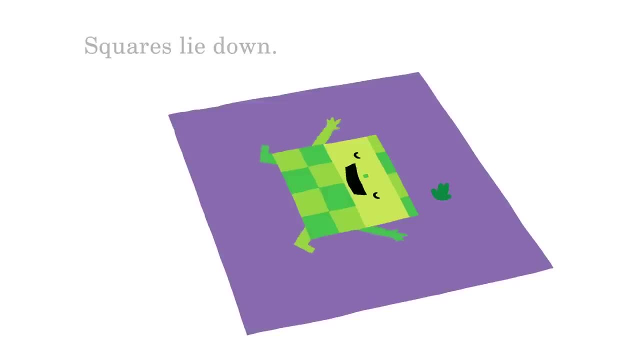 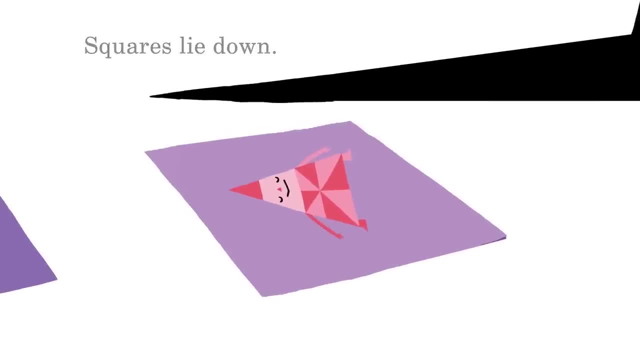 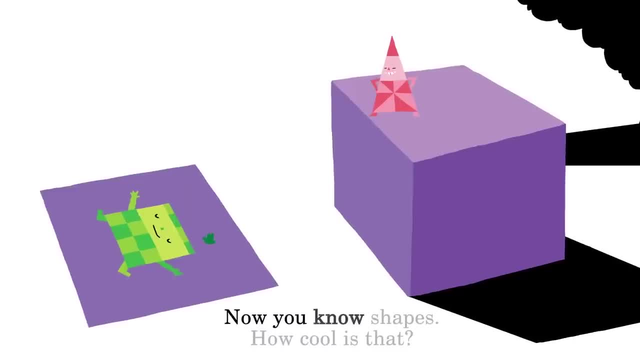 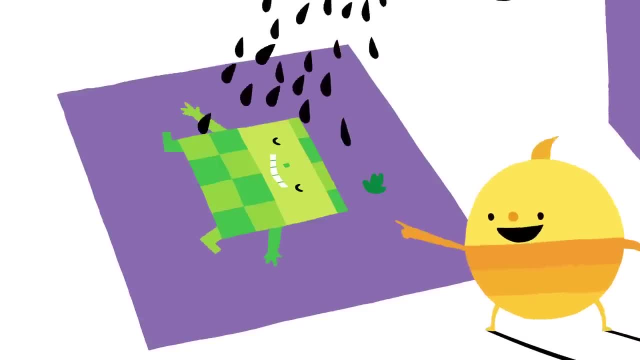 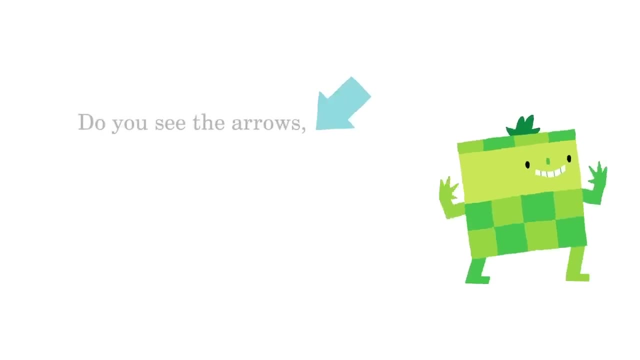 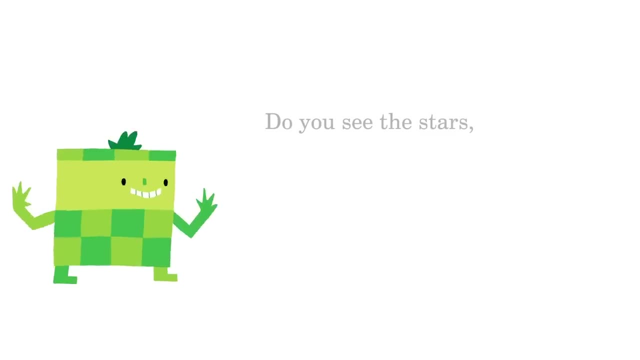 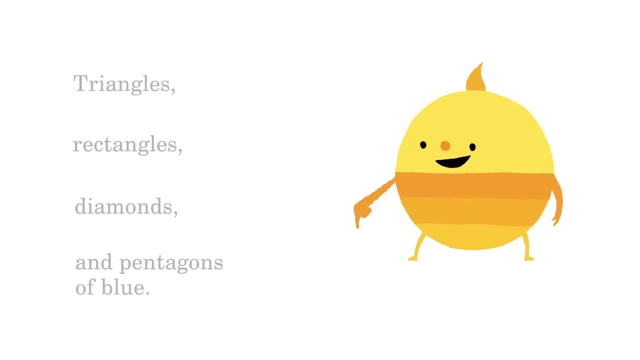 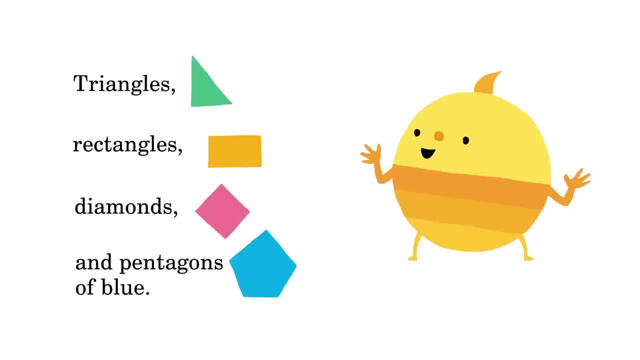 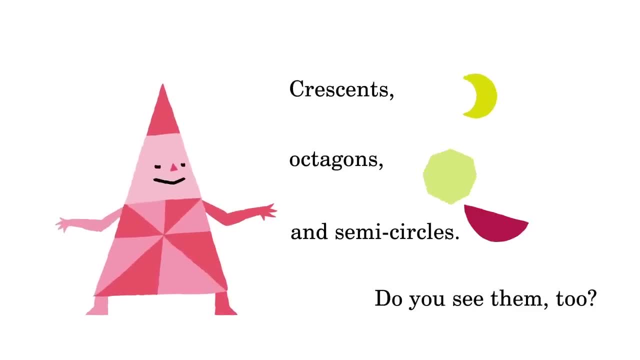 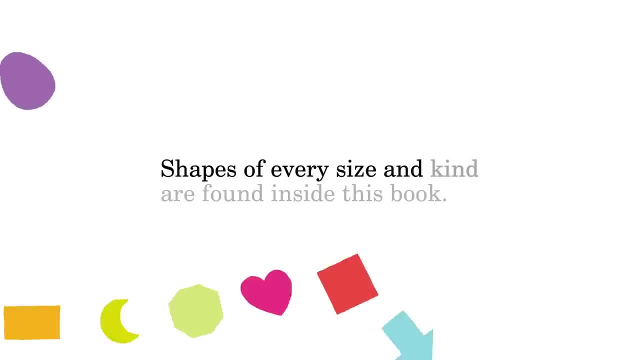 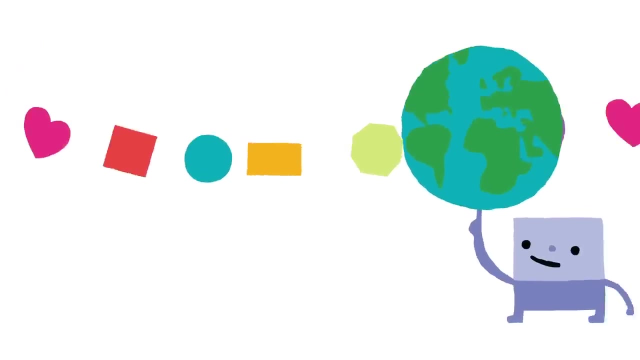 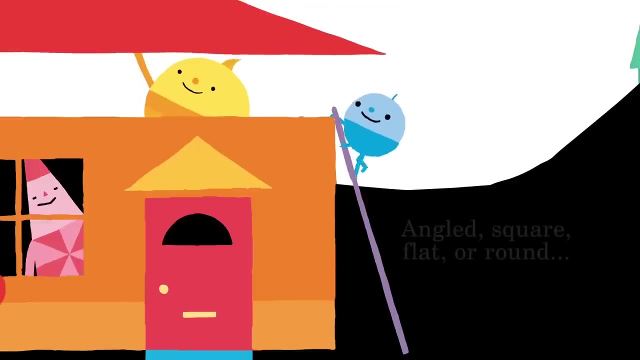 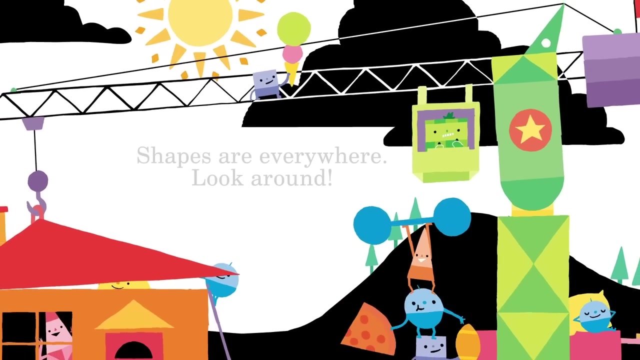 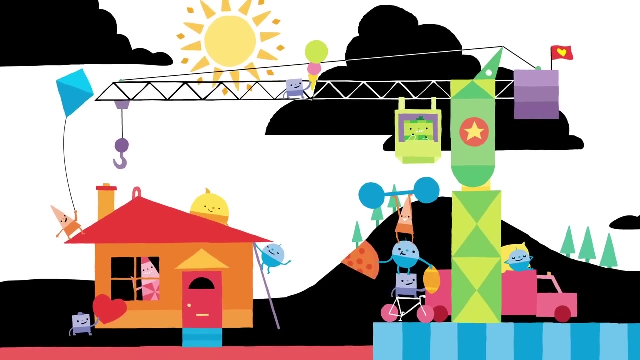 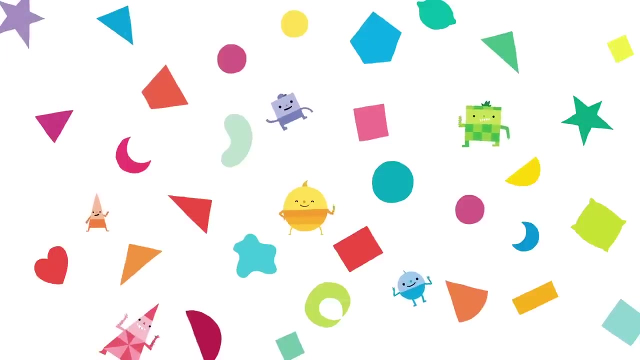 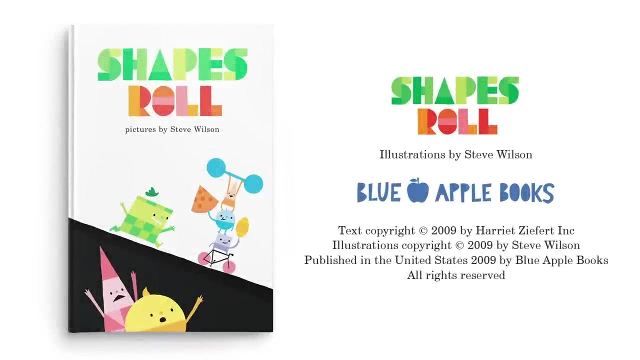 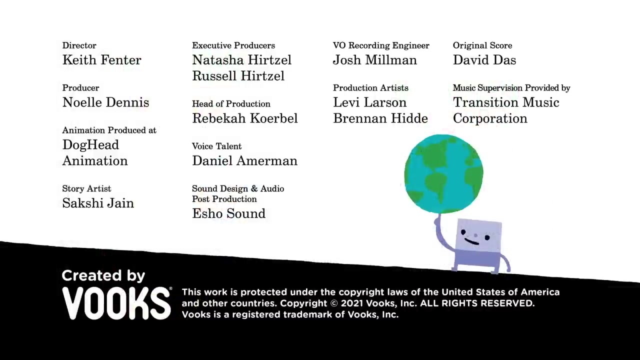 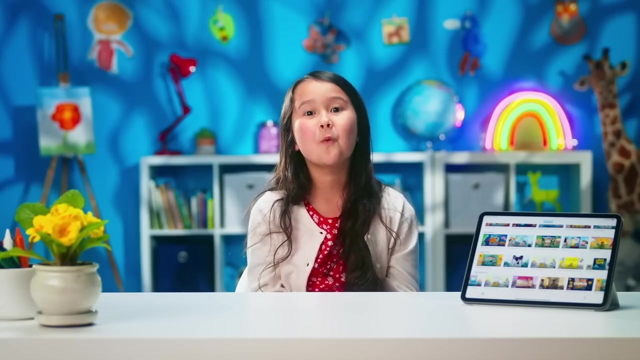 Do you see them too? Shapes of every size and kind are found inside this book. The whole world is made of shapes: Angled, square, flat or round Shapes are everywhere. Look around. If you don't have books, what are you waiting for?